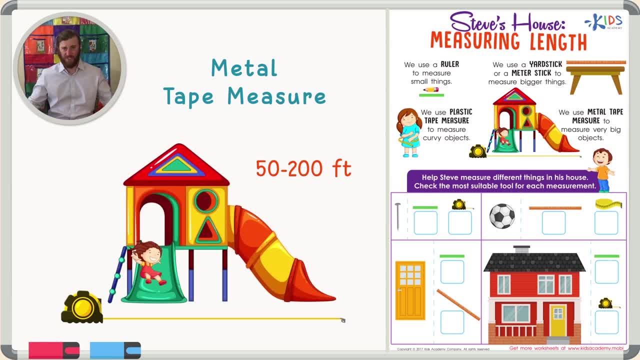 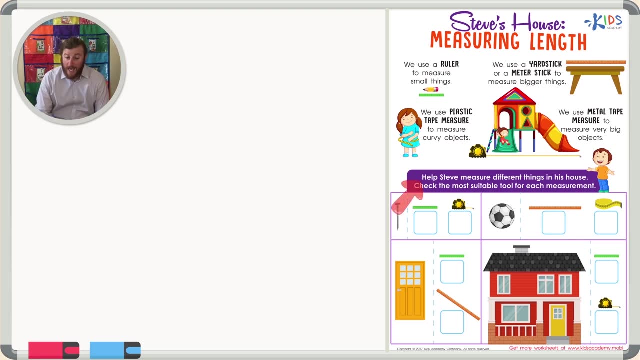 tape measure. It measures objects that are three feet long, meaning it can measure things like houses and cars. A metal tape measure is really big for measuring things that other tools can't measure. Now let's read the directions for our worksheet and get started right away. Help Steve measure. 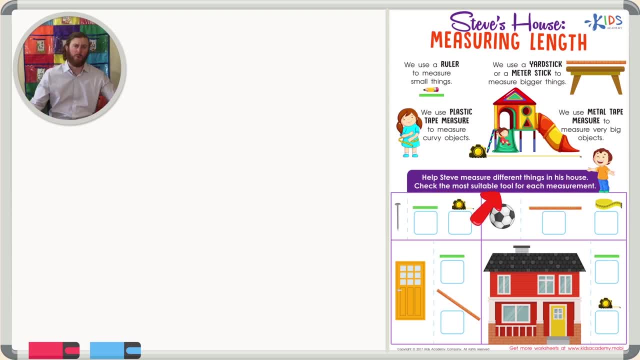 different things in his house. Check the most suitable tool for each measurement. Let's get started First. we have a nail and our two choices for measurement are a ruler, a ruler and a yardstick- A ruler or a metal tape measure. Now I remember telling you that a metal tape measure can measure. 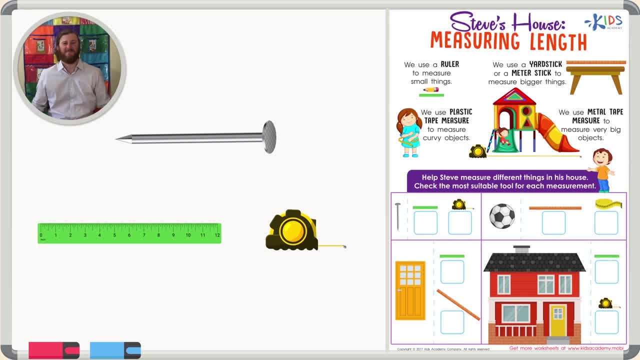 distances between 50 and 200 feet. Is a nail really that big? I don't think so. In my estimate, or my best guess, I would say: nail. a nail is a few inches long, So the best tool to measure a nail is in. 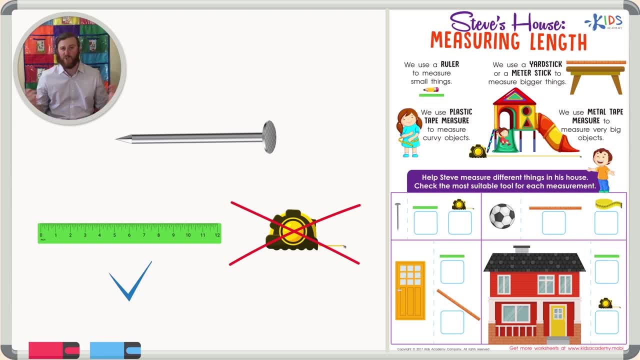 fact, a ruler. We would only need one ruler to measure a nail, which makes this the right choice. The next object we want to look at is a soccer ball, and I can see for this measurement we want to measure around the soccer ball. So really to measure an object that's curvy or a round object. 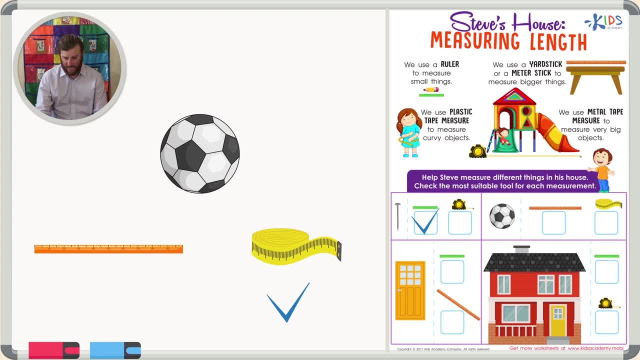 there's really only one choice: that we talked about The plastic tape measure because that will help us measure curvy or imperfect objects. A ruler would not be an appropriate choice for this, because there is no straight line to measure on a soccer ball, The next object we want to measure or choose. 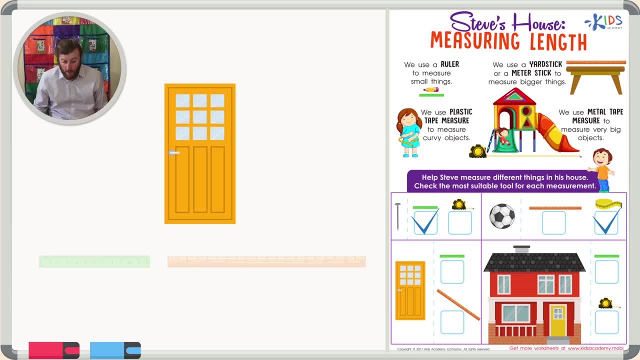 the correct tool to help us measure is this door. Now, this door is pretty big, so I don't think a ruler is going to be enough, because we're going to have to use multiple rulers to measure this door. But if we had one meter stick, I think we might be able to measure this door. We might need two, but 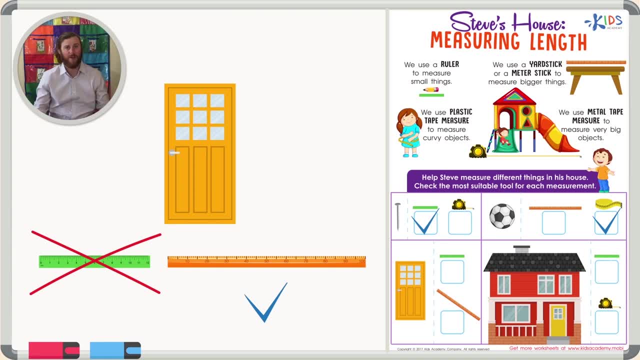 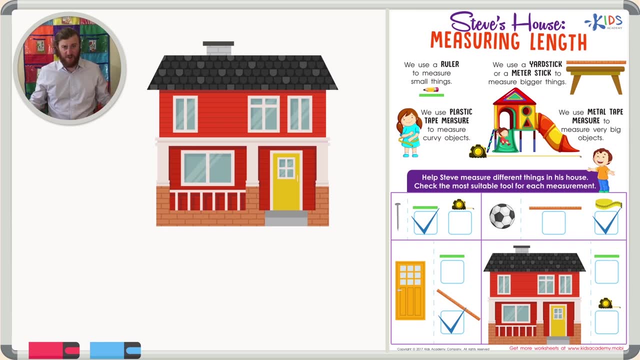 still, it's more appropriate than using a ruler to measure the door, So let's choose the meter stick. Finally, we have a house. How big do you think this house is? Pretty big. Our two choices for the house are the ruler and the tape and the metal tape measure. If I were to measure this house using the ruler, I would need a. 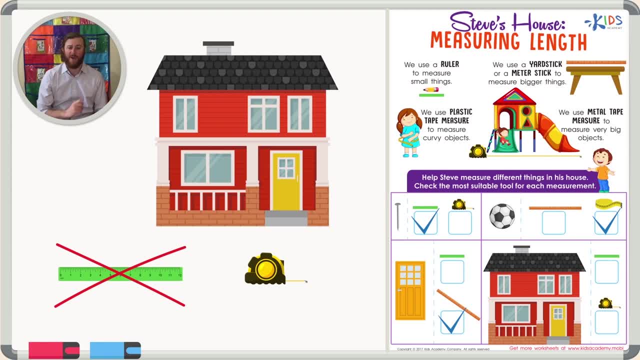 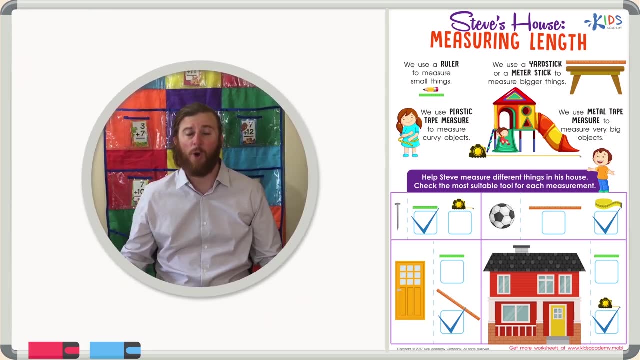 lot of rulers, But if I were to measure just using one metal tape measure, I might be able to measure the whole house. So the metal tape measure is the appropriate choice here, because it can measure distances or lengths from 50 to 200 feet long. Thanks for watching boys and girls, and I hope you. 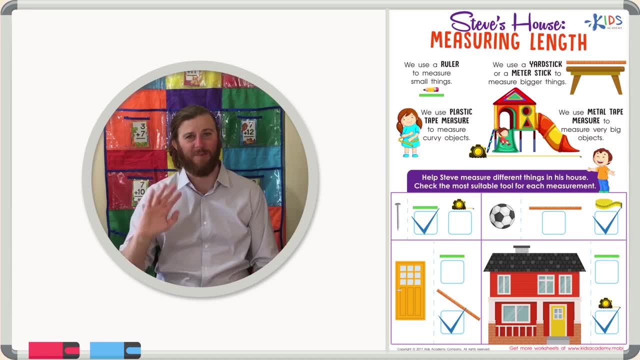 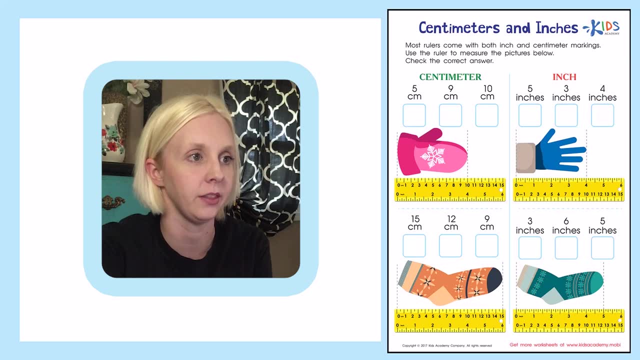 learned a little bit about selecting the correct measurement tool. We'll see you next time. Hello, I have a new worksheet today. The name of the worksheet is called centimeters and inches. Most rulers come with both inches and centimeter markings. Use the ruler to measure the picture below: Check. 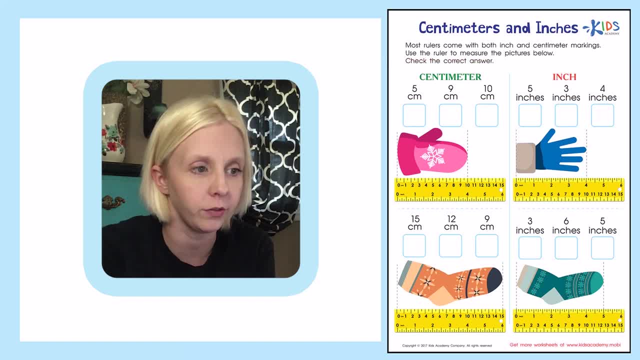 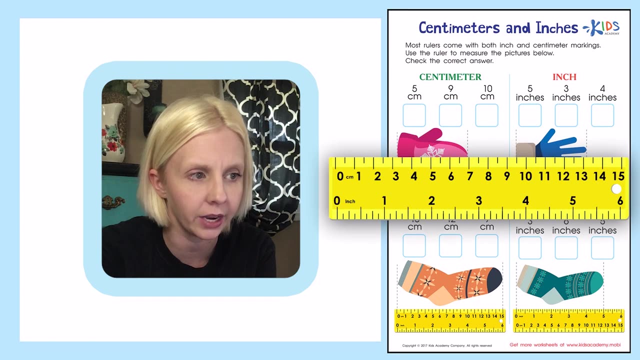 the correct answer. So what we're going to be doing is we've got all of these different things here, and to measure those different things Now let's look and kind of look at our ruler first and kind of get an idea of where everything is. When I look at this ruler, I see that these little ones are. 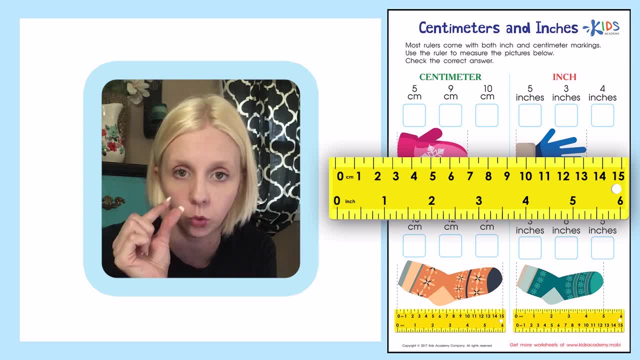 all going to be the centimeters. The centimeters are kind of the smaller ones that are really close together and the inches are a little bit bigger. The inches are a little bit wider. So these are the inches down here. We're going to take a look at this. We're going to look at our options. 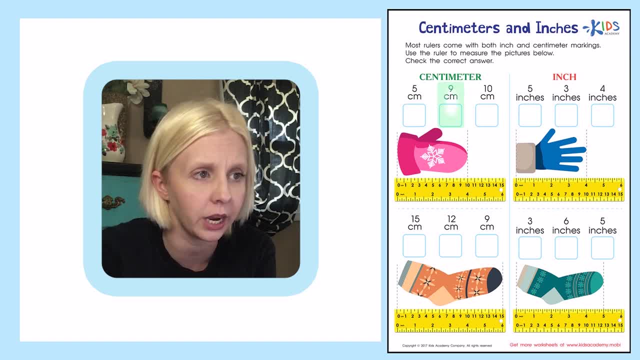 And it says we either have five centimeters, nine centimeters or ten centimeters. So we're just looking at centimeters right now. So we're going to come down here and we're just going to pay attention to the small numbers. These are these numbers right up here. We don't want to. 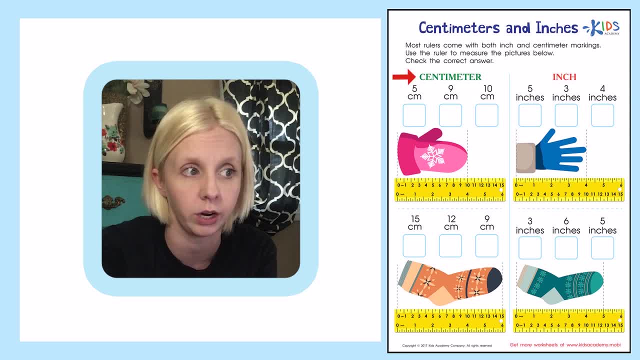 get confused down here with these. We're just looking for a centimeter answer, Okay. so let's look at the glove. We're going to always start at the end of the ruler, Okay, and we're going to measure it or line it up with the end of the ruler, and then we're going to come down here and we're 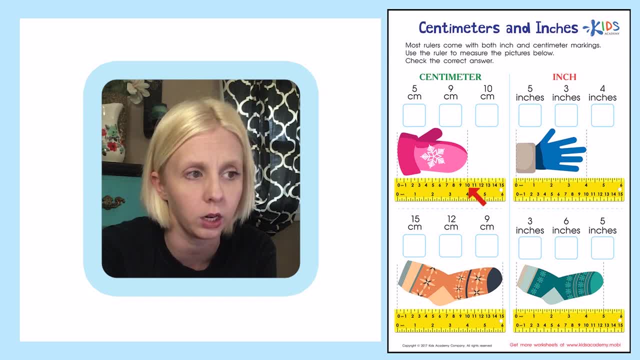 going to measure where it stops. And it comes right down here and they've drawn out this little dotted line for us to show us where it ends, And it looks like it's going to be right on the 10.. So I'm going to come up here and I'm going to check the correct answer it said. So I'm going. 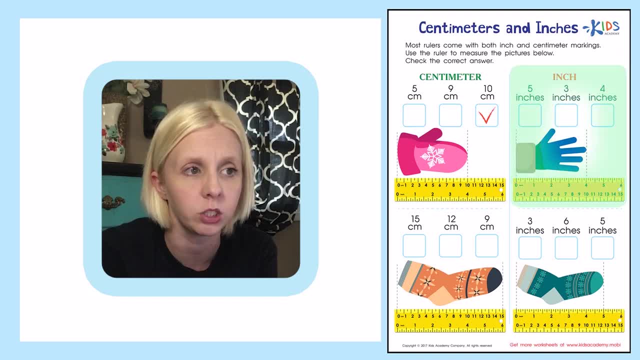 to put a check right here for 10 centimeters. Okay, let's go into the next one. That was pretty easy. This one even says up here in red it's inches. All our choices are going to be inches, So now we're. 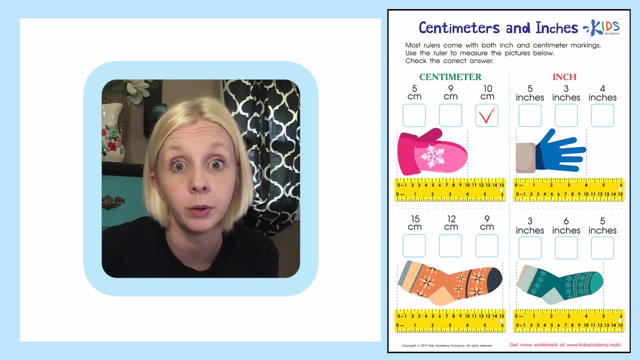 no longer looking at the small numbers, We're looking at the big numbers. But don't be confused. They kind of went to trick you on this one, I think, and they switched them up over here. The centimeters were on this side, but but now they're down at the bottom. So up here now, closer to the 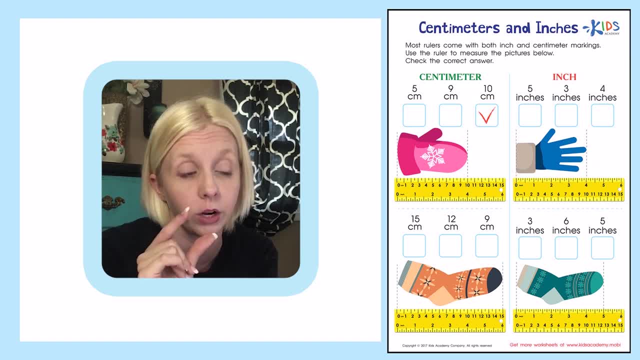 glove is the inches, So we're looking for those ones that are wider, The bigger numbers. Okay, we're looking for inches. So let's see, We've lined up our glove at the end of our ruler. We come all the way down here And where does that last little part of our glove go to? It goes to: 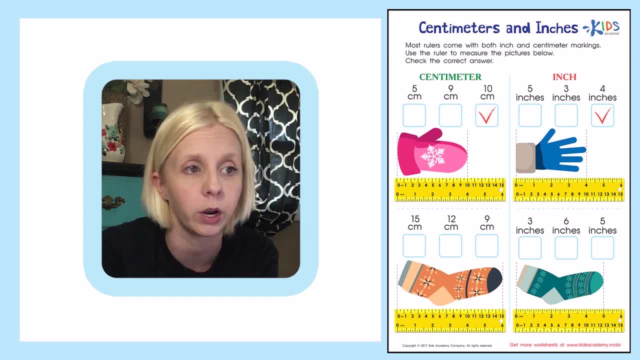 the four. So it's going to be four inches, and four is right over here, So I'm going to put a check right on that one. The next thing we're measuring is a sock. Look at that sock. We're going to come over here and we're going to measure the sock, And this time we are also looking for 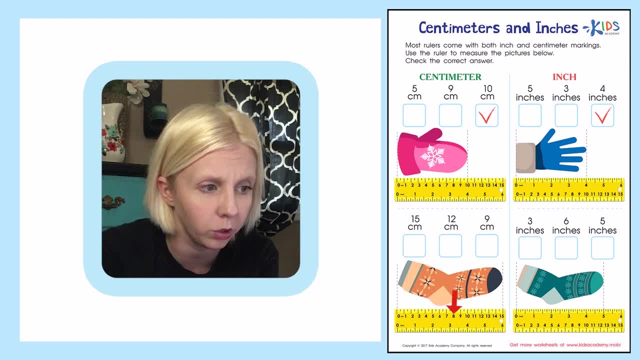 centimeters. Okay. so centimeters are the little numbers, So little numbers. they've got right next to the sock for us. We're going to. we've got our sock lined up at the end of the ruler. We're going to come all the way down and it is lined up right over here. So it is going to be 15 centimeters. So 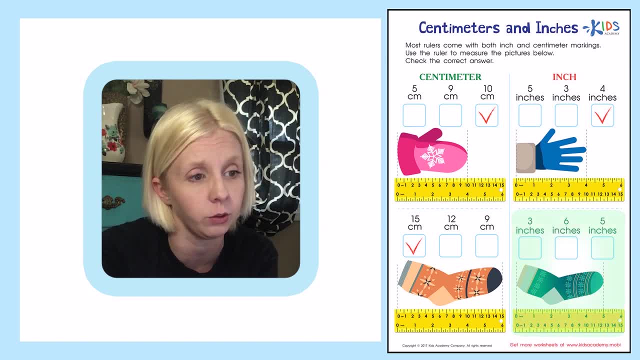 there on the 15.. Our last one is another sock. We've got a blue sock. this time It's a little bit smaller, Might be a kid's sock- And we are looking once again for inches. Okay, and the inches are the big numbers And they're already right over here on the end or closest to the sock. 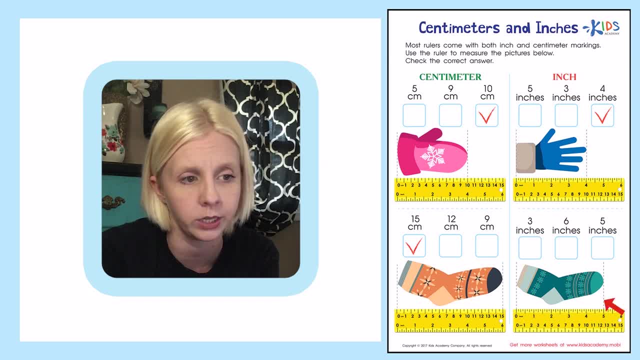 We've lined up our sock with the end and we're going to measure all the way down. And where does it come to? Our dotted line is going right to the five, So it's going to be five inches. I'm going to put a check right there. Measuring is so much fun and it's pretty. 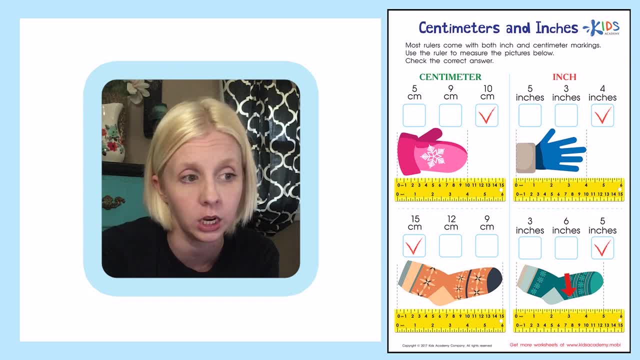 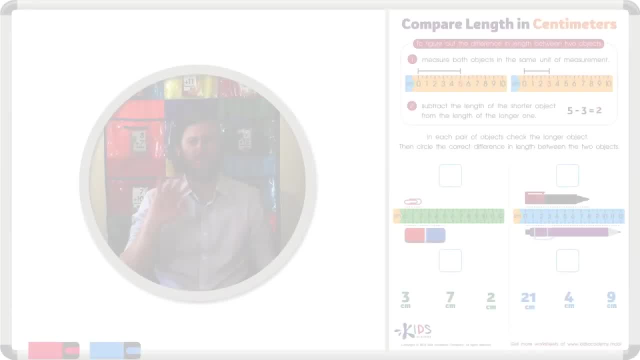 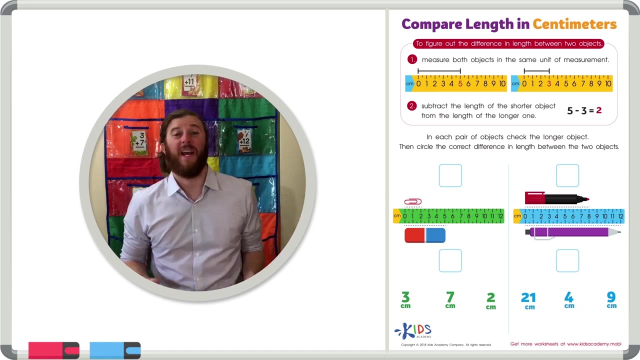 easy, isn't it? You just have to check, You have to measure and look and see where everything is lined up. But we did it today. Nice job. Hello, boys and girls, This is teacher Mike, And today I'd like to talk to you about comparing the length of objects in centimeters, Meaning we're going to 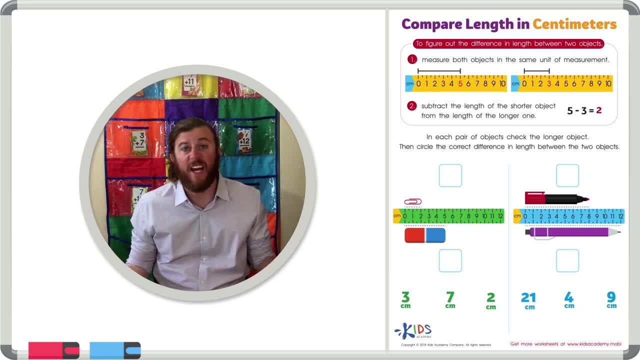 take two different objects and see which one is longer, And then we're going to see how much longer that object is. So let's talk about a strategy for accomplishing this. So to figure out how much longer one object is than another object, First you have to measure both objects. 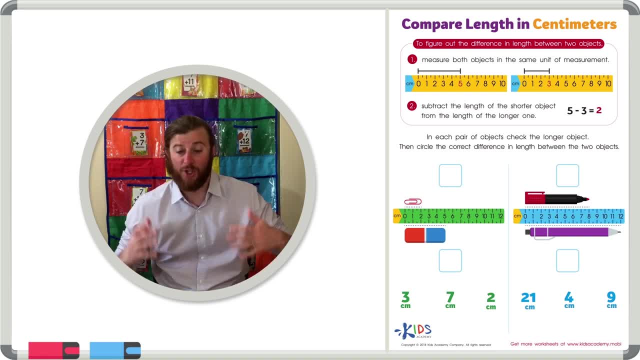 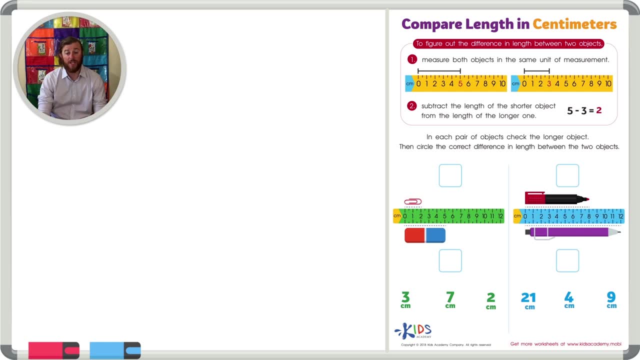 Then you'll take the length of the shorter object and subtract it from the length of the longer object. So let's look at an example. Let's say we measured two different nails. The first nail we measured was five centimeters long. The second nail we measured was three centimeters long. Well, 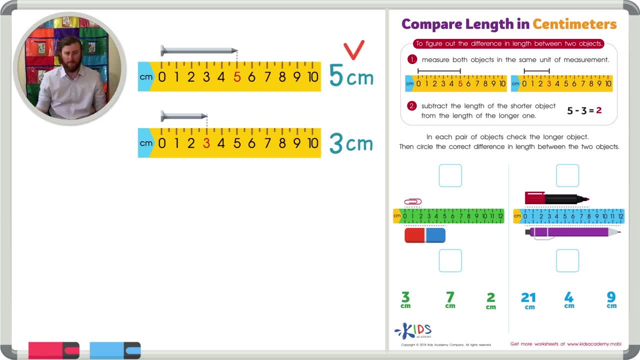 it's easy to tell that the five centimeter nail is longer, But how much longer? Well, we can subtract to find out. We always put the bigger number or the longer object up top and the shorter object up below. So let's subtract. five minus three, We subtract. 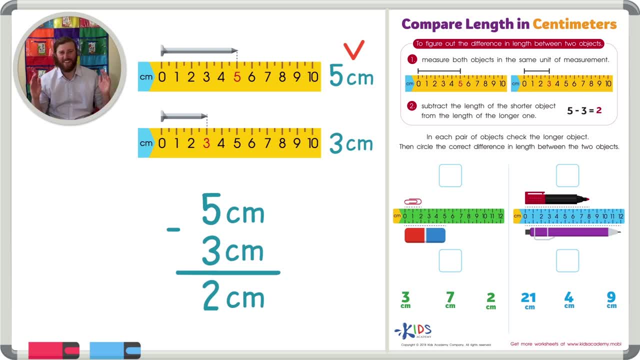 five minus three, we get two. So I know the difference in length between these two objects is two centimeters, And we found this out through subtraction. Let's read the directions for our worksheet and get started right away, And let's use this strategy to help us to complete the 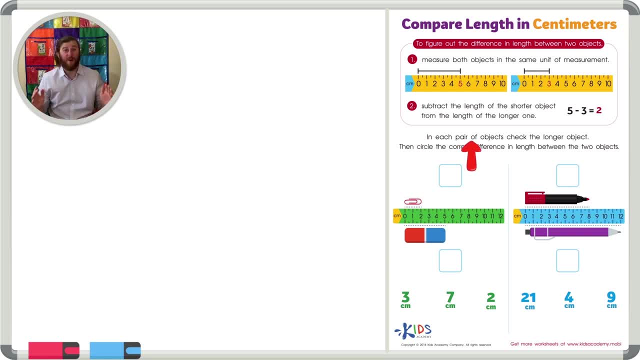 worksheet. In each pair of objects, check the longer object, Then circle the correct difference in length between the two objects. Let's look at our first two objects. We have a paper clip and an eraser, So let's look at the length of the paper clip. The paper clip starts at: 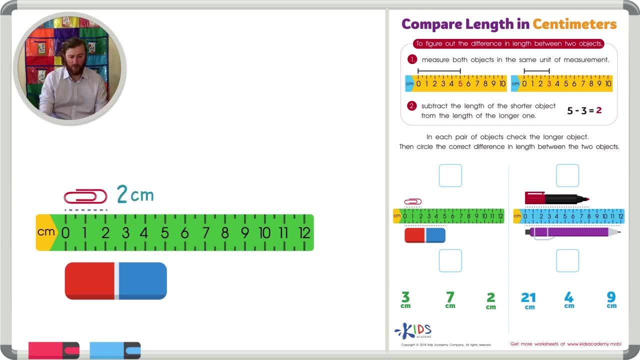 zero and goes to two centimeters. So we know our paper clip is two centimeters long. What about the eraser? If we look closely at the eraser, we can see the eraser is 5 centimeters long. Now we have to rearrange. 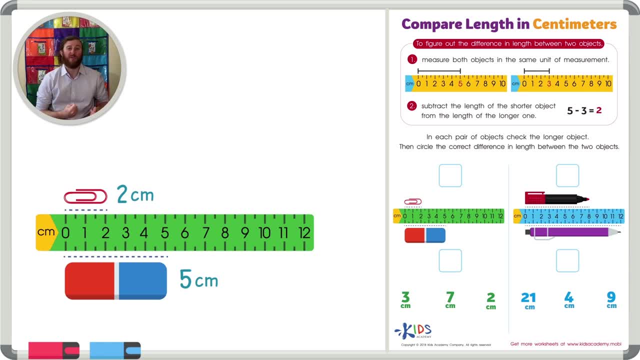 these numbers. so the bigger number is on top. so that way we're subtracting the shorter number from the bigger number. So let's switch these numbers. We'll put 5 on top and subtract 2 away from 5.. What is 5 minus 2?? Well, it's 3.. So the 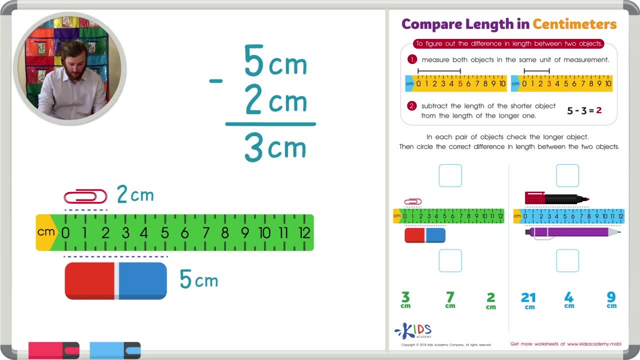 difference in lengths is 3 centimeters. So now let's go ahead and fill in our worksheet. We know the eraser is bigger because it's 5 centimeters long. That's bigger than 2 centimeters, for sure. How much bigger is the eraser than the paper? 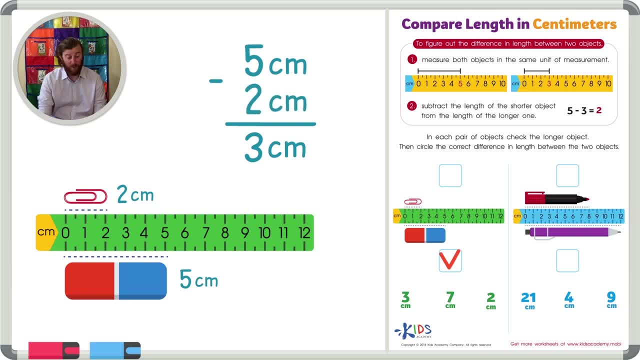 clip. When we subtracted the length of the paper clip from the length of the eraser, we got 3 centimeters. So we know that the difference in length between the two objects is 3 centimeters. So let's go ahead and circle 3.. Let's take a. 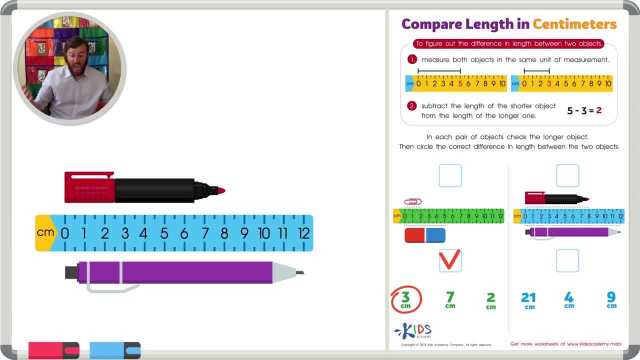 look at our next two objects. We have a marker and a pen. Let's see how long the marker is. Well, if we look closely again, it starts at 0.. The marker goes from 0 to 8 centimeters long. So let's mark down that our marker is 8 centimeters long. But what? 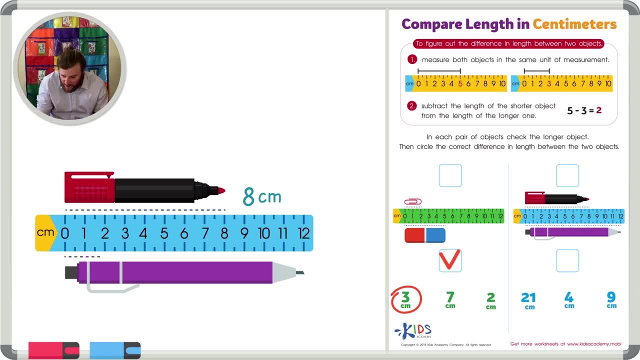 about the pen. How big is the pen? The pen starts at 0 and goes all the way to 12.. What is the difference between the pen and the marker if the pen goes to 12 centimeters? Well, again, we're going to have to flip these numbers to find out. 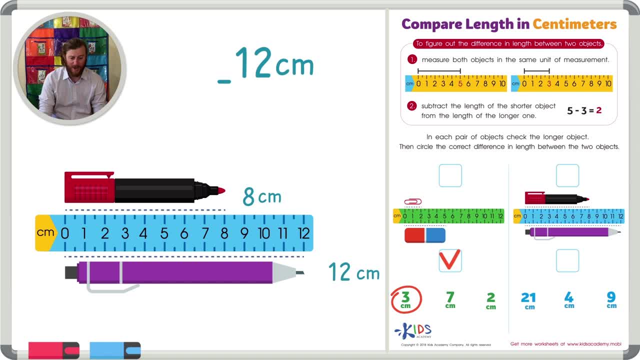 So let's put 12 on top, Then we'll subtract 8. We can count up from 8 to 12 to find the difference between 8 and 12.. Let's go ahead and do that: 8,9,10,11,12, So the difference is 4. 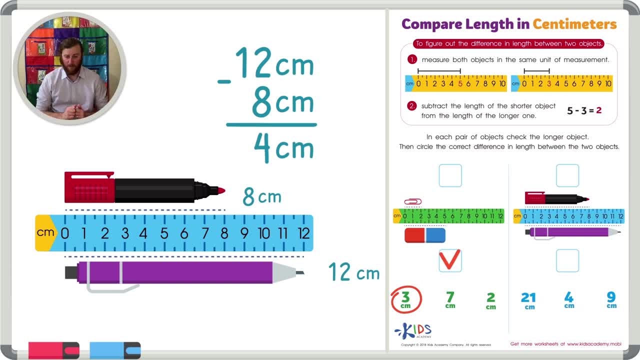 centimeters. so let's go ahead and fill in our worksheet now. So just by looking at the two objects and using the ruler, which object is bigger? Well, of course the pen is bigger. So let's go ahead and check the pen Now: how much bigger or how much? 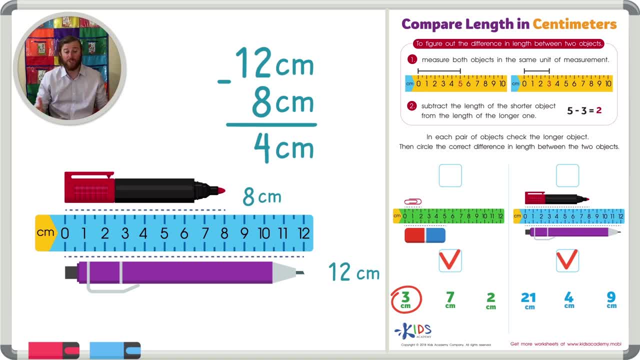 longer is the pen than the marker. When we subtracted the shorter object from the longer object- 12 minus 8, we got a difference of 4 centimeters. So we know that our pen is 4 centimeters longer than our marker. Let's go ahead and. 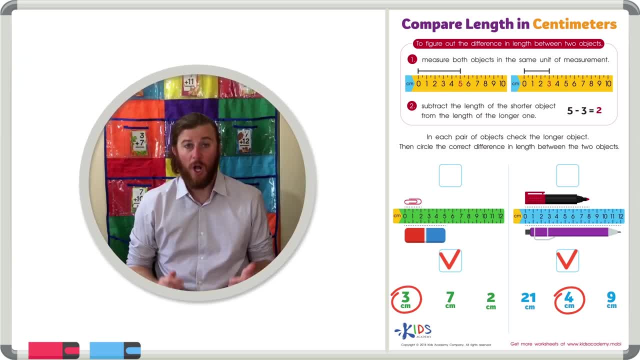 circle 4 centimeters. Remember boys and girls. when you want to find the difference in length between two different objects, first measure both objects, then subtract the length of the shorter object from the length of a longer object. The difference in the length of these two objects will tell. 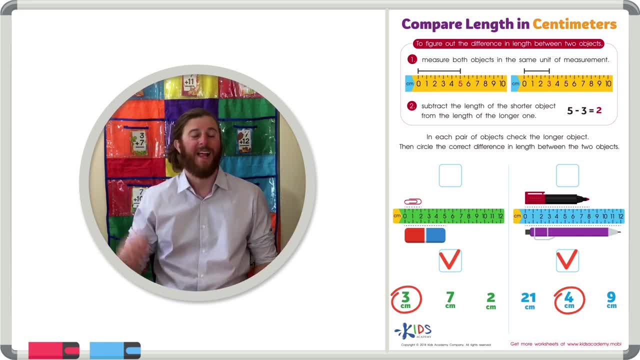 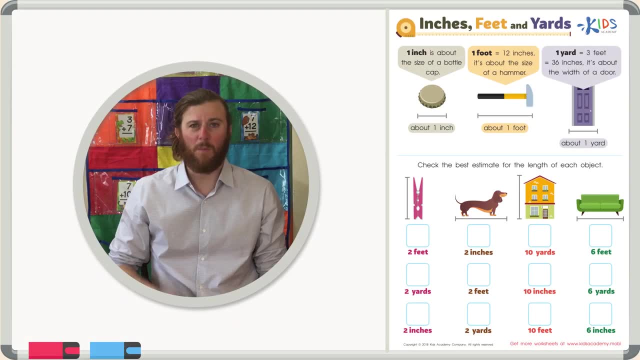 you how much bigger one object is than the other. Thanks for watching, boys and girls, and we'll see you next time. Hello, boys and girls, this is teacher Mike, and today I'd like to talk to you about estimating measurement. Now, this is kind of tricky, but it can also be kind. 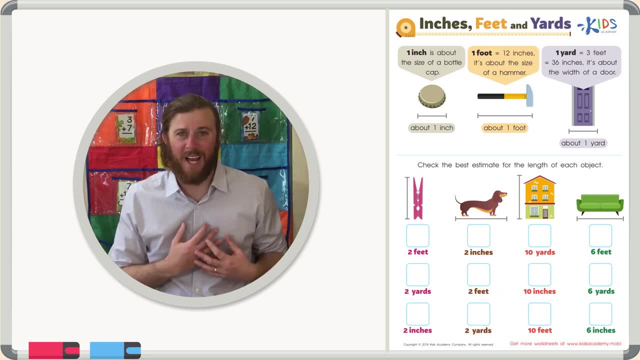 of fun. If you can use references from your own life to make estimates or good guesses about sizes, estimating could become a lot more easy and even fun. You can point out different objects in the world and guess the sizes based on your reference estimates. So let's go over what some good estimates for some. 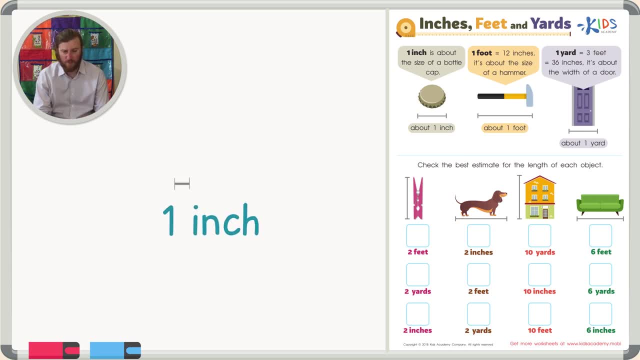 different sizes are. Let's first talk about one inch. One inch is the size of a bottle cap like you pop off the top of a soda- An really, really small. can you think of some other things in the world around you that are about one inch? let's talk about one foot. a foot is about the size. 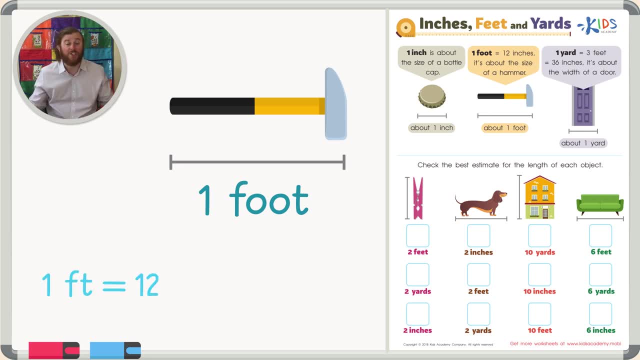 of a hammer. now, a foot is 12 inches long, so it would be like putting 12 bottle caps next to each other, but that's not really a good estimate. can you think of other objects that are about the length of one foot? a hammer is a good. 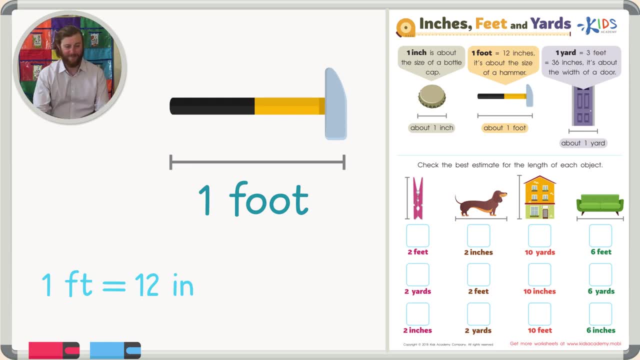 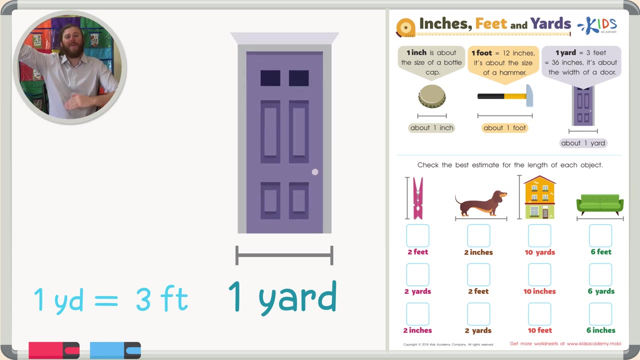 suggestion, but what else can you think of? the last measurement that I'd like to go over is one yard. a yard is three feet long. now, a good estimate for a yard is about the width of a door, not the height, because you need adults to get in the. 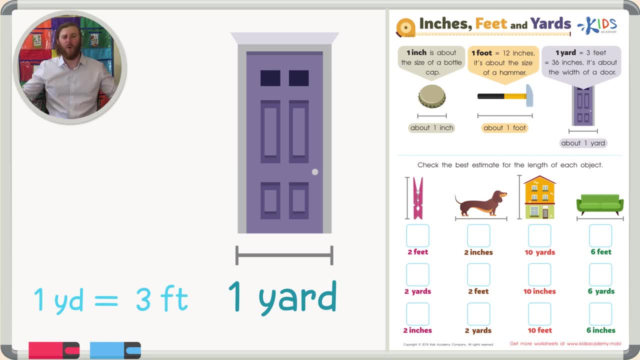 height of a door, so that's going to be more than six feet long. the width of a door, meaning how wide it is or how long it is, is about three feet long or one yard long. so when you want to estimate one yard, think about the width. 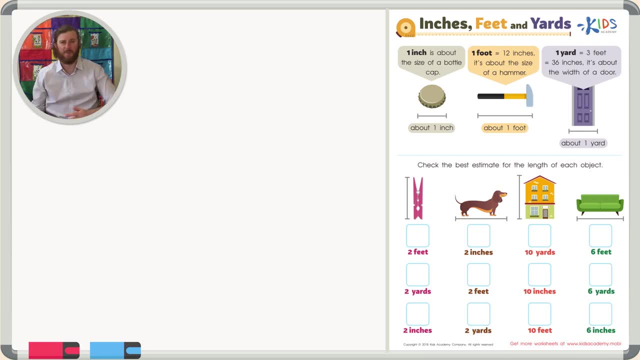 of a door. now let's use these estimates to help us answer the questions below. let's read the directions in inches, feet and yards and get started right away. check the best estimate for the length of each object. okay, first we have a clothespin and it wants to know the height or the length of this clothespin. 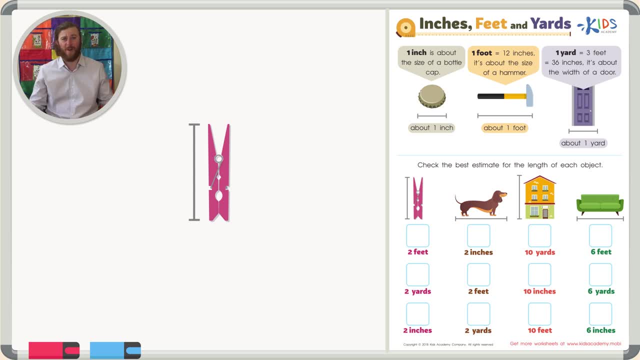 it's marked off very nicely for you and it's going to tell you the length of this clothespin and it's going to tell you the height of this clothespin and maybe a foot or something like that. now let's look at the size of the clothespin. 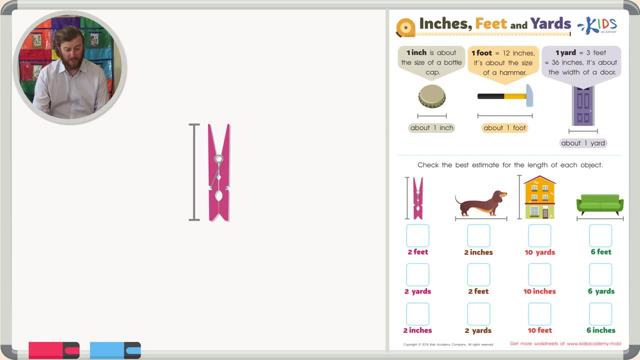 and we don't want to get too rid of the WHEEL DISTANCE, but we're going to make sure that we're looking at it nicely for us. so let's look at our answer choices and choose the most reasonable guess. so our first answer choice is: 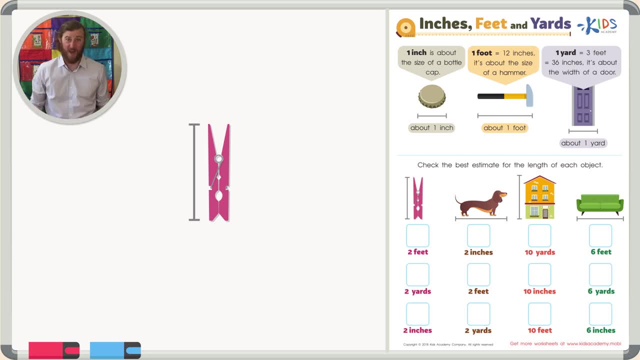 2 feet. now think about the size of a clothespin. Now think about 2 feet. that's like two hammers put right next to each other. Is a clothespin the size about 2 hammers? The clothespin is way smaller than two hammers. that can't be the right answer choice. 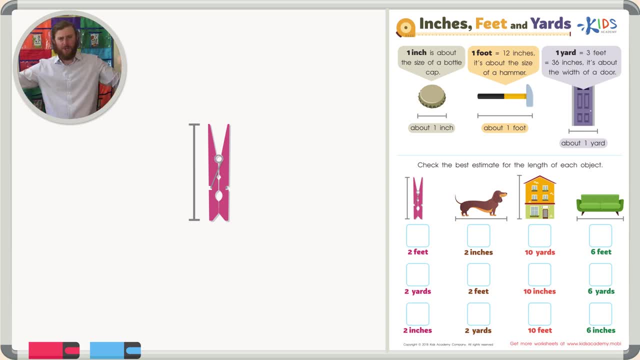 because that's even bigger. that's like the width of two doors, and a clothespin is tiny compared to that. finally, we have two inches or two bottle caps put right next to each other. does that make sense of the size of a clothespin? I think so. 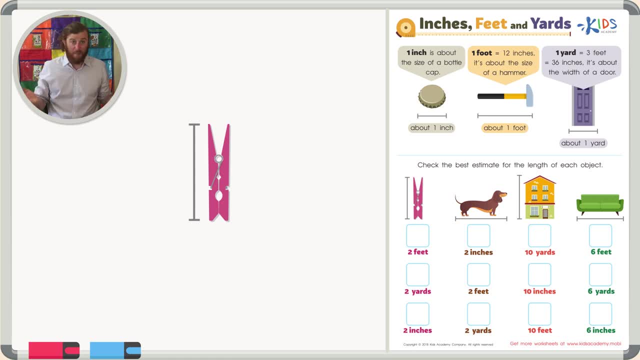 now is the clothespin exactly two inches? it might be, but it also might not be. but it's very close and that's why we call it an estimate. it's like a good guess. so two inches is the correct estimate for our clothespin. let's take a look at our 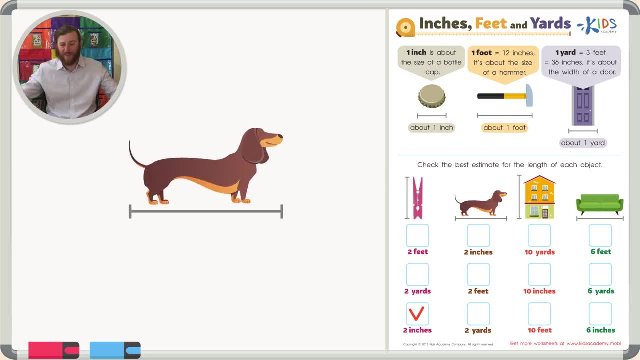 next object: a dog. we want to know the length of this dog. well, let's look at our answer choices and see if we can make sense of this. our first answer choice is two inches. two inches is gonna be way too small, because that's just like two bottle caps put right next to each other. I have never seen a puppy. 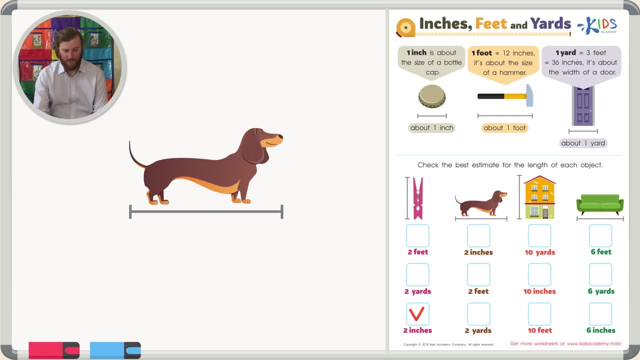 that small, even a brand newborn puppy. two feet now. that makes sense, a little bit more sense. can you imagine two hammers put right next to each other? that is about the length of the dog. so i think that is the correct estimate. but let's look at our last answer. 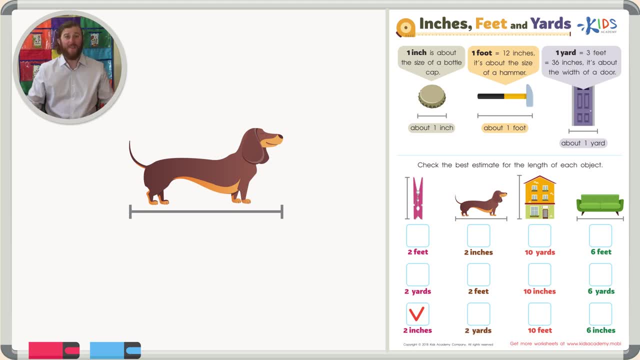 choice. just to be sure again, it's two yards. that would be like the width of two doors put next to each other. that would be one huge dog. so i don't think that's the correct answer choice. the correct answer choice is two feet, because the length of a dog is about the length of two hammers. 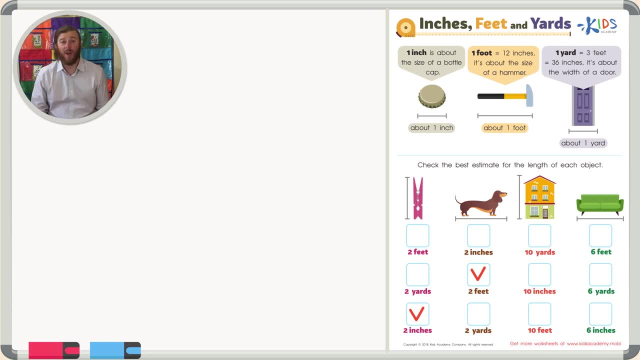 next we want to know the estimate for the height of a house. now, that's going to be really big. so our answer choice of 10 yards already seems to make sense to me. but let's look at our other answer choices. just to be sure: 10 inches, is your house as tall as 10 bottle caps put on top of each.